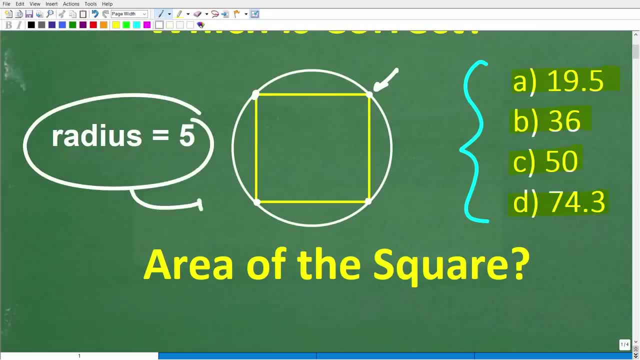 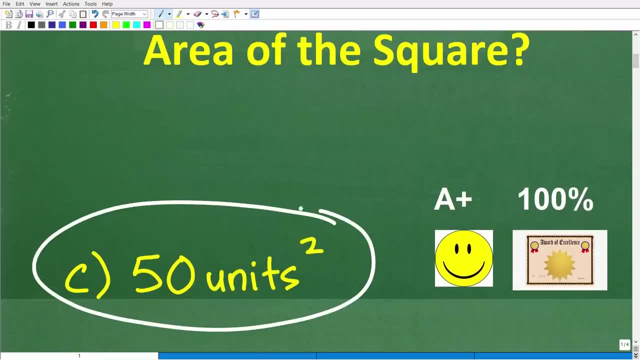 All right. so once again we have a square and a circle, and the radius of this circle is 5.. So what is the correct answer? Well, the correct answer is C, which is 50. And we are talking about area here, so we're going to have to throw in this units squared. 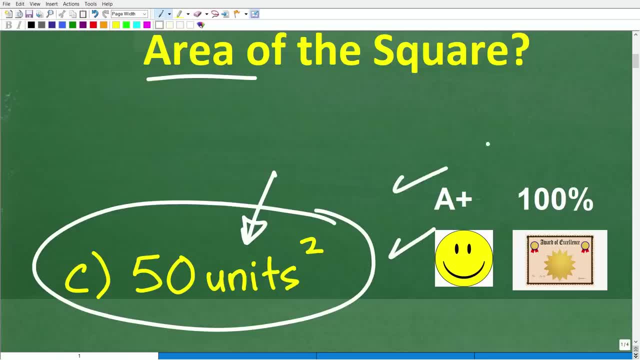 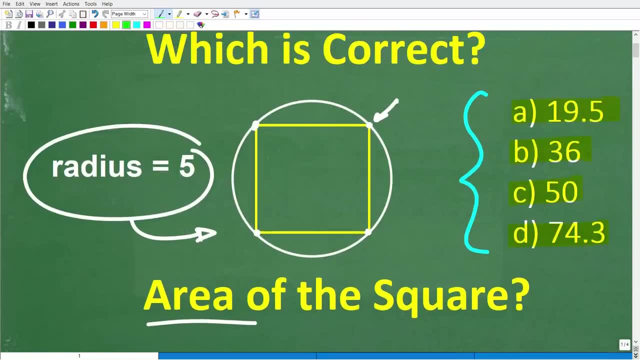 Now, if you're able to figure this out, you definitely get a happy face and a plus a 100% And a certificate, And a certificate of excellence for being able to solve an interesting little math problem that involves a square and a circle. 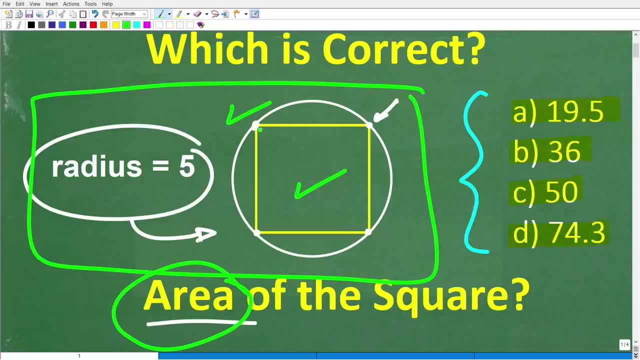 So if you know a thing or two about the area of a square and the area of a circle, well that could very well be enough to solve this problem. But actually there's another component to this problem that really kind of unlocks the solution. 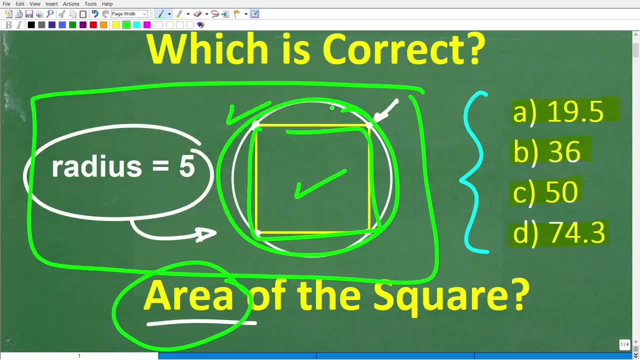 So if you're like really struggling, you're like I don't see the solution, Mr YouTube, Math Man, Well, again, this is not going to be That difficult, But let's go ahead and get started now. And here is our problem. 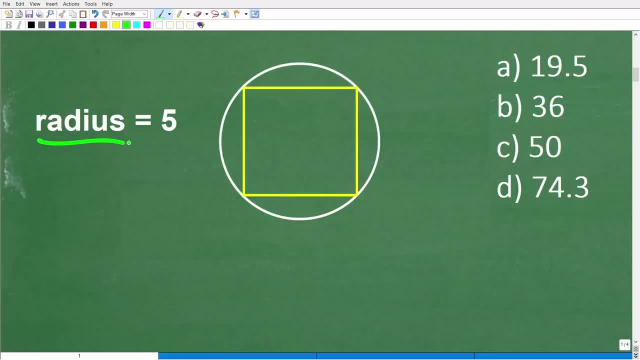 So first of all, we need to understand what the radius of a circle is, right. So if we don't know what the radius of a circle is, well, we're not going to be able to understand the problem. So I'll explain this in a second. 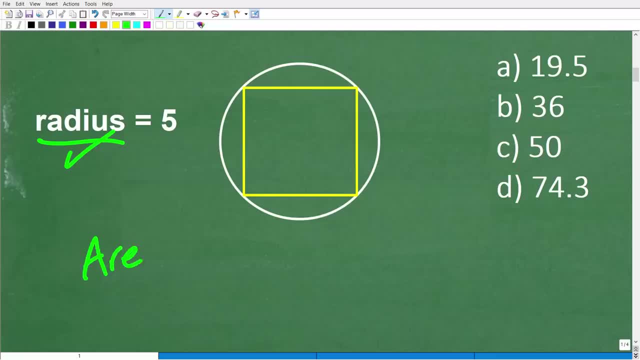 Now we are talking about the area We want, the area of this square. So we're going to need to understand the formula for the area of a square right, And we have. So let me ask you, do you think we need to also need to know the area of the formula for the area of a circle right? 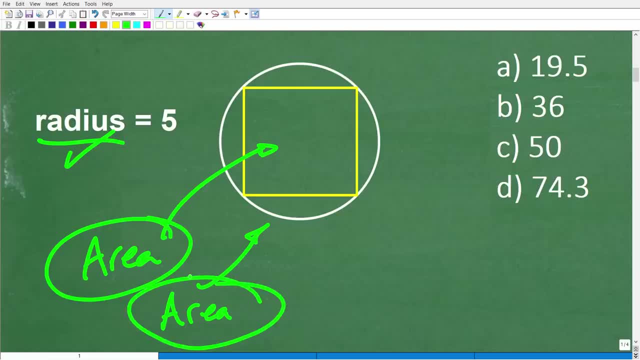 We definitely need to know the formula for the area of a square, But what do you think about the area of a circle? Are we going to need that as well to solve this problem? So, really, what we need is a strategy, right? So you're thinking to yourself: well, how can we find the area of this square? 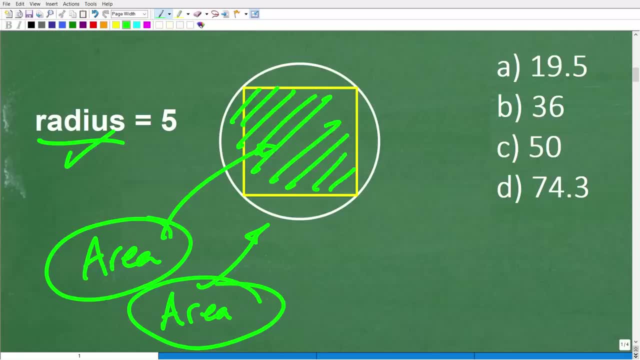 Right? Well, there's a couple of different ways we can kind of go about doing this, But the simplest way is to know the formula. But once we understand the formula for the area of a square, we're going to need to get the information. 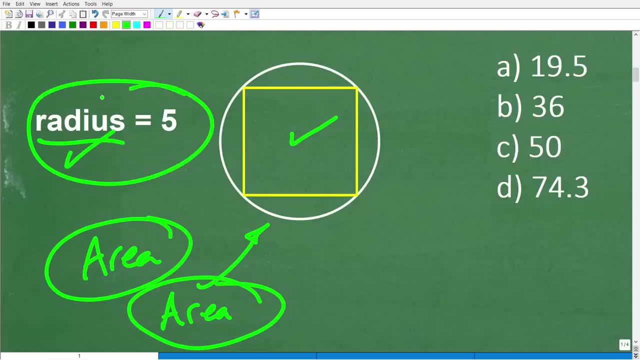 Right, But we have a lot of things here to discuss, And the first is: what is the radius of a circle? Now again, this is a multiple choice question And if you encountered this on a test or a quiz, and as long as you're not getting penalized, right. 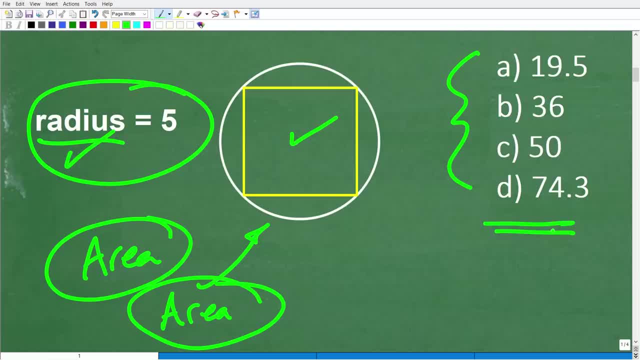 you always take a guess, even if it's like it's a random guess. right, Be like I don't know. I'm feeling pretty Lucky with 36 today. Unfortunately it's wrong, But at least you didn't leave the question blank. 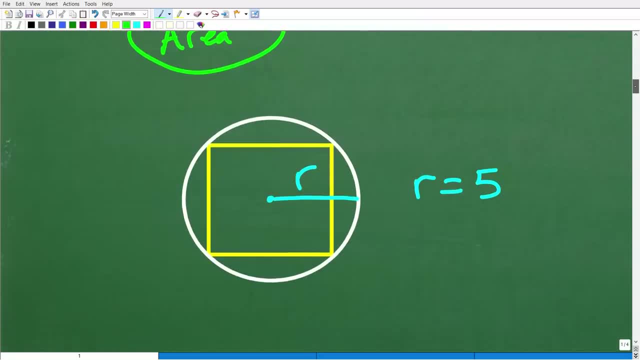 All right. So let's go ahead and get into this right now And let's talk about what the radius of a circle is. All right, So the radius of a circle is the distance from the center of the circle out to the edge. 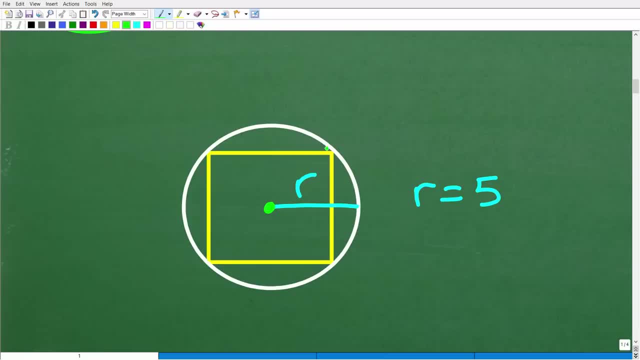 Right. So here we're seeing the radius And, of course, we have our lovely square right here. So the radius is five. And there's another word that you need to know when it comes to circles, And that's it. If we have two radiuses like this forming one line, this entire width of the circle is called the diameter. 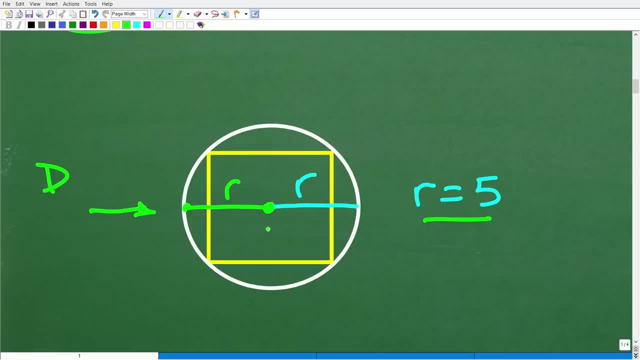 Right So the radius emanates from the center out to the edge And it goes in all directions Right. So this is the radius, That's the radius, This is the radius, And this is the radius, et cetera, et cetera. 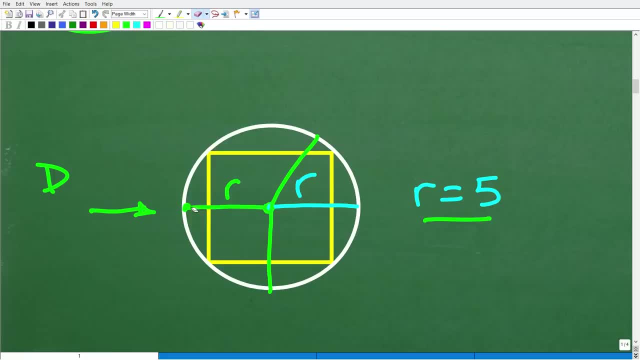 So it's the same number. All right, Now I've kind of given you a little bit of a hint for those of you that might still not kind of see how to figure out the information that we need about this square, Right, Right. 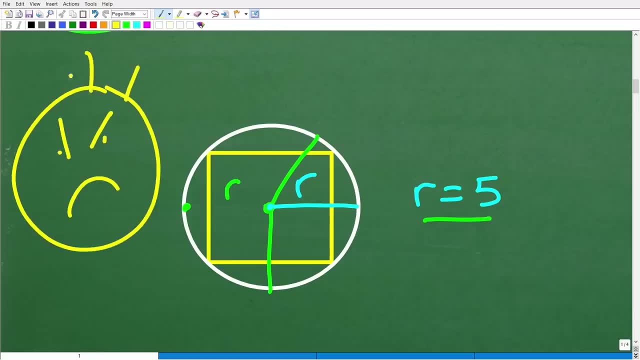 So you're like, I'm a student of math man, I know what the radius is. But again, this particular problem has my hair standing straight up. How do we find the information? Well, we're going to talk about that right now. 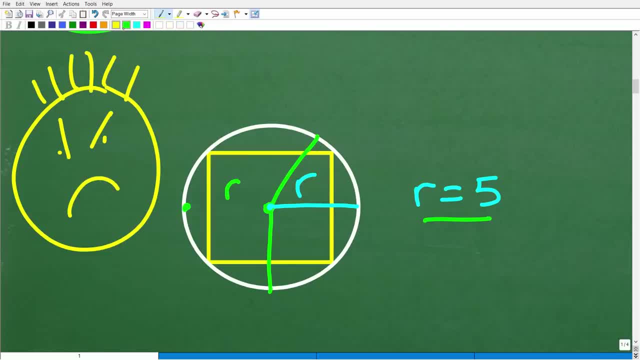 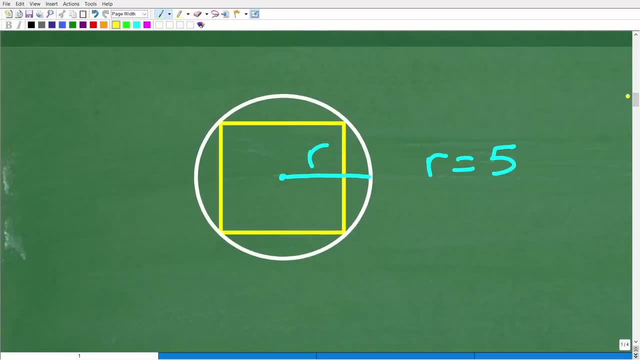 And when you see how we're going to get the information about this square, you're going to be like, wow, that wasn't that difficult, All right. So again, here is our scenario, And we need to figure out something about this square. 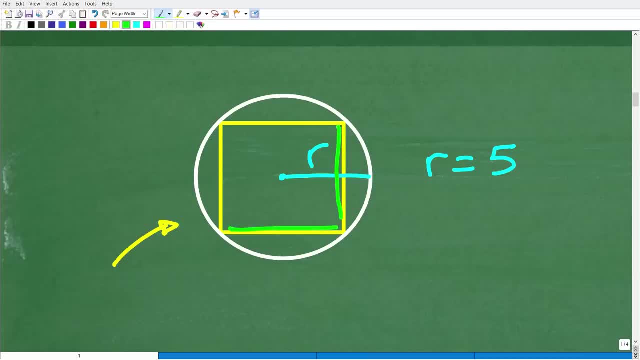 Now the best thing is the actual lengths of the side. All right, Now. this is a square, So that's the first thing that we need to understand is: a square has equal sides. A square also has right angles, like: so. Now there's another thing about squares that are really, really important is that the diagonals of these squares right here intersect at the center. 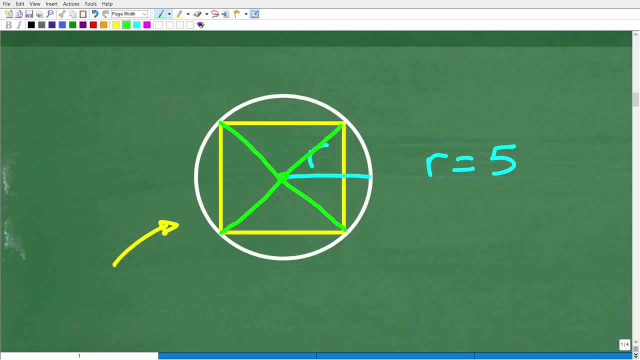 Okay So the diagonals of this square is also the center of this circle. Okay So, hopefully this was something Now you know kind of, can visually assume, but that is the case, All right, So we have a square. 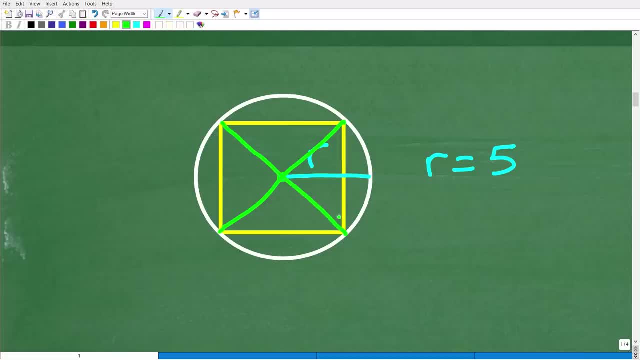 The diagonals of this square also go through the center, which, of course, is the starting point of the radius. Okay, So again, the radius is five. So how can we get some information about this square? Well, I'm going to show you right now. 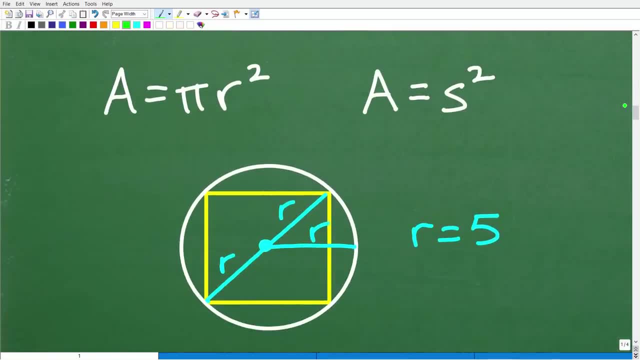 All right. So here is our two formulas about the area of a square, which is a side square, And the area of a circle is pi r squared. Now I'm just kind of Showing you these formulas, but really what I need to show you is this: 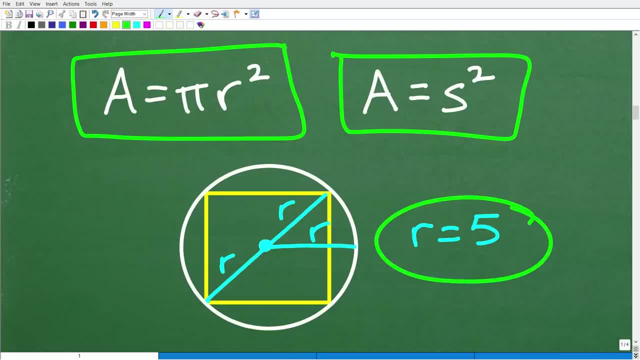 Okay, So here is our square inscribed in the circle. Now, when you think of the radius, a lot of you probably were thinking in terms of this, or maybe you had your radius going this way. but also, okay, we can kind of form the radius from the center along the diagonal of the square. 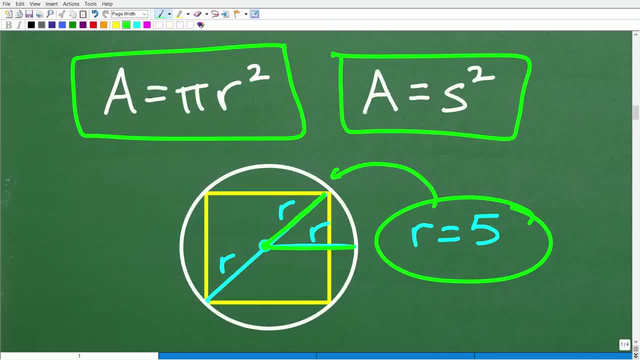 Okay, And if you kind of visualize it this way, this right here is the radius, That's half of the diagonal, Meaning That from here to here is the whole width. This is the diameter right, So it's two radius. 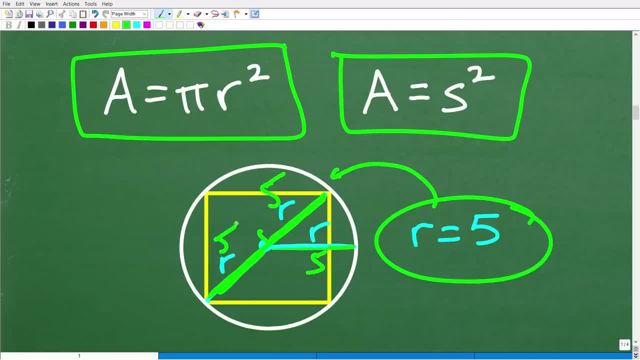 So this is five, Okay, Cause the radius is five and this is five. Well, we have a right triangle right here, because this is a square, and a square has, by definition, a 90 degree angle. So, really, what we have is a lovely right triangle with the hypotenuse, this right here being 10.. 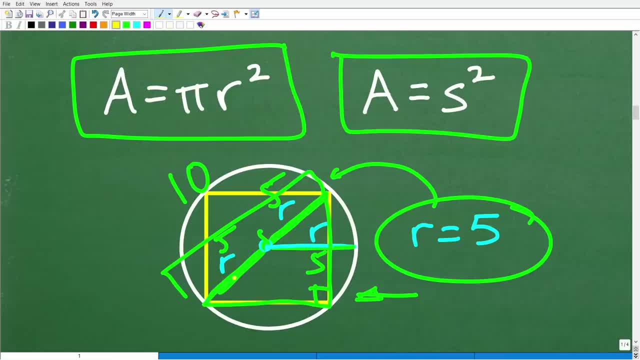 So very, very interesting. So, if we can figure out, uh, let me kind of uh raise this here for a second. effectively, what we have right in here is a right triangle. right, It's a 40, poor right triangle, but the hypotenuse, uh, the distance along this diagonal is 10.. 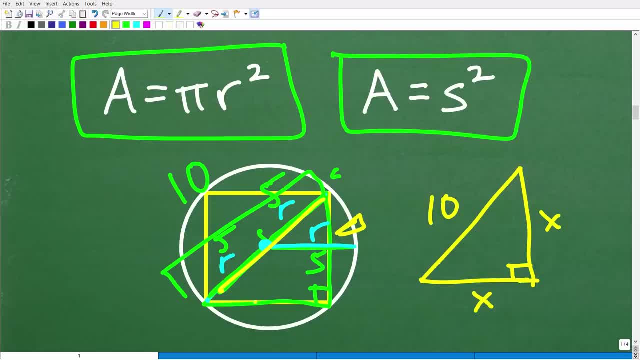 Now, we don't know the sides of this right triangle, but if we do find the sides, we can easily calculate the area of the square, because the area of the square is side squared right, In other words. or You know, whatever the sides are, they're the same. um measurement of a square, just square it. 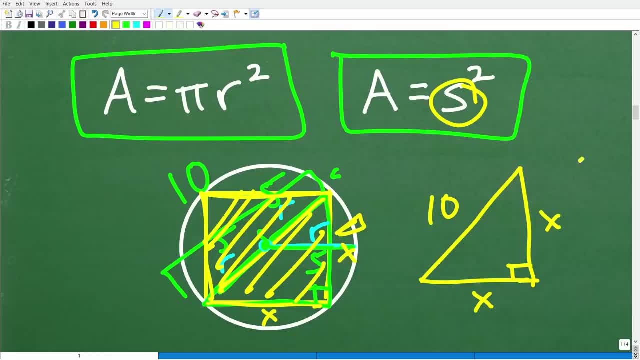 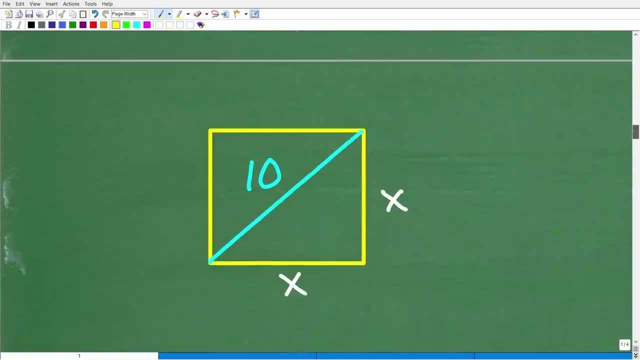 Uh, and we have the area of the square So effectively. this is the information that we have, So how can we figure this out? All right, So here's what we really have. Okay, So the radius again, uh, starts right here, from the center of the square. 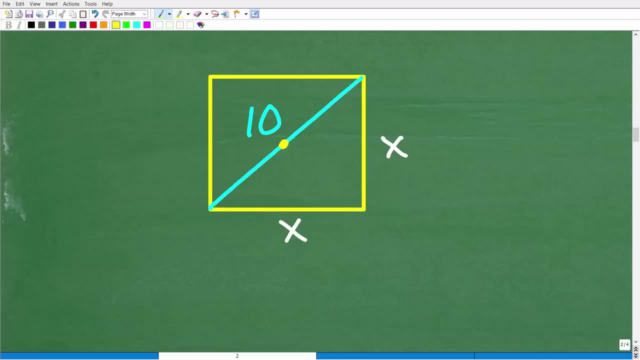 So the center of the circle and the center of the square are the same position. That's kind of more or less it right there. So here's five. Here's five. That's the radius. So, uh, what we need to do is find the area of this square. 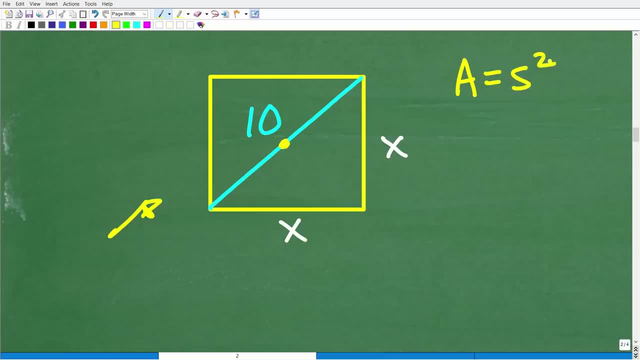 All right. So what's the area of this square? Well, the area is equal to side squared, and we don't know the side, so let's just call it X, All right. So that means that the area of this particular uh circle or this particular square is X squared. 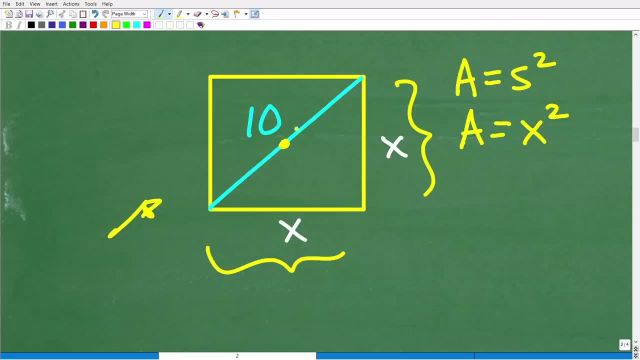 All right. Well, how's this going to help us out? Well, we do know again that the diagonal is 10 and this is a right triangle, Okay. So this triangle over here is the same thing, Okay, As this triangle right here. 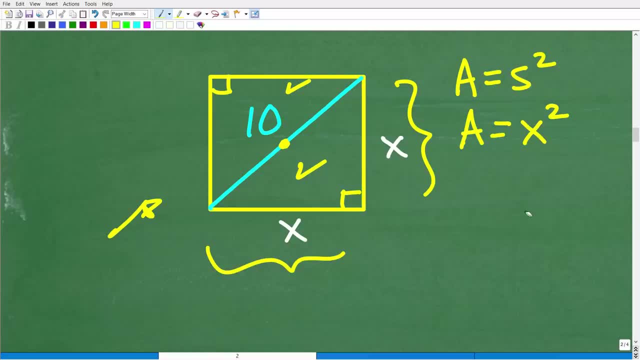 So do we have enough information? Actually, let me kind of draw this way, uh, to figure out the side. Okay, With the right triangle, uh, this being X, this being X, it's the same thing, And this being 10.. 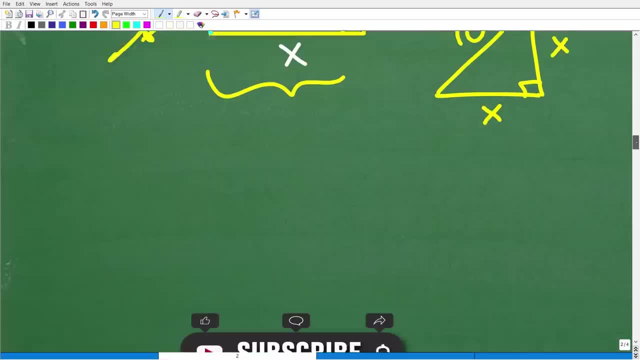 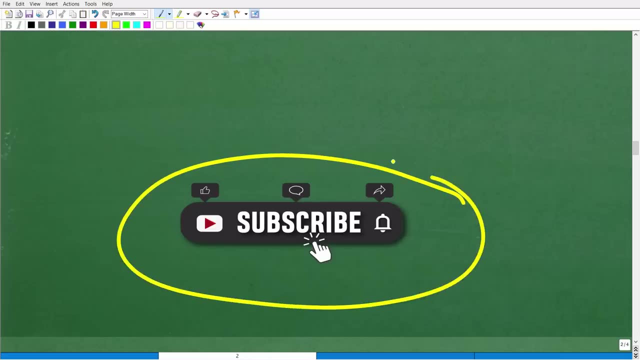 Well, indeed, we do. All right, This is not going to be that difficult, especially if you understand the Pythagorean theorem. but we're going to get to that in just one second, But first I need to show you this, which is an invitation to support this channel. 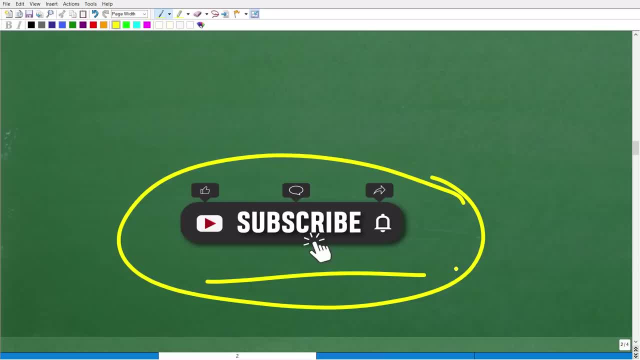 Now, what's this channel all about? Well, it's about math, obviously, but uh, really, uh, what I try to emphasize, um, um, this particular channel, is that anyone could be successful in math. Okay, It's just not about me showing you how to do a bunch of math problems, because a lot 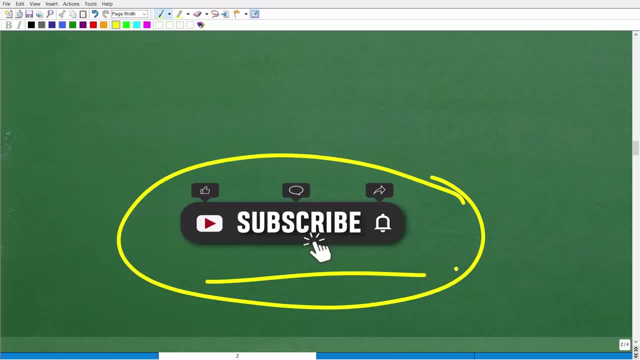 of you are like: yes, yes, that's what I do all day. I watch my teacher solve a bunch of math problems. but if you're frustrated and you're like I don't get how to solve math problems, I don't understand. Mr YouTube math man. 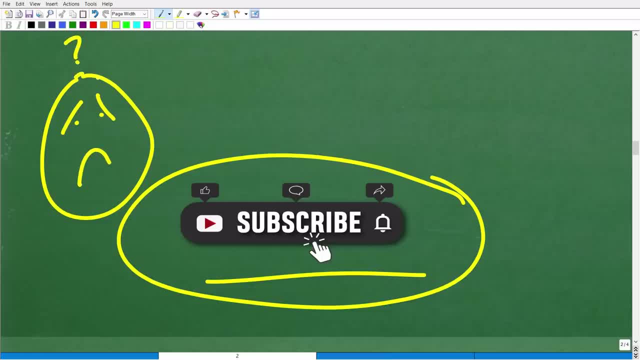 Well, this is what this channel is about. It's about encouraging people to not give up on math And really, uh, to kind of um communicate a positive message that really needs to be heard more and more and more is that people can be successful in math, right. 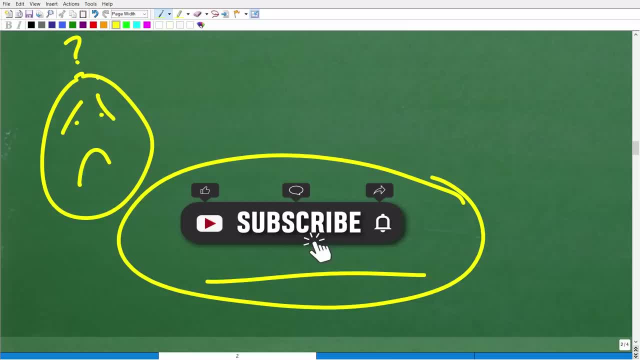 Uh, there's no such thing as somebody who's like, oh, naturally terrible at math. right, It takes work, It takes time, So don't give up. And, most importantly, it takes, uh, you know- instruction that you like and understand. 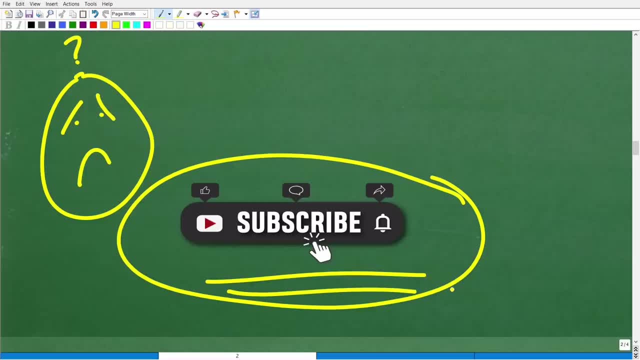 So if you need help in mathematics, check out my full main math courses. You can find links to those in the description of this video. Also, I have like 3000 plus math uh videos on my YouTube channel, So check those out and make sure to hit that notification bell as well. 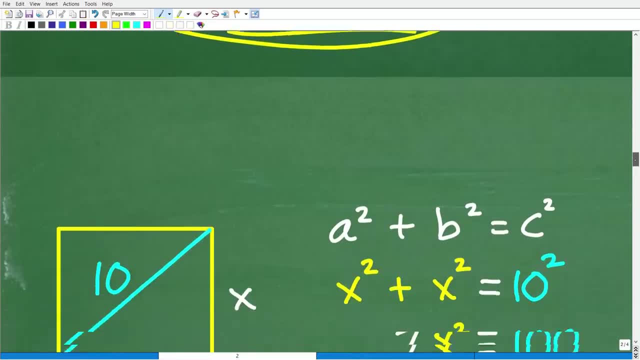 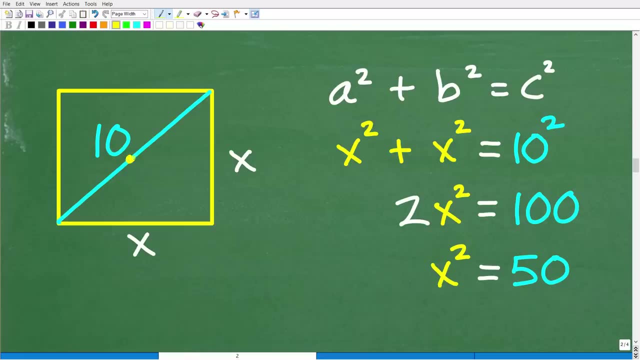 So you can get my latest videos. All right, So let's get back to this problem. So now that we know, uh kind of the situation here is our inscribed uh square And uh this is the center of that circle and we have a radius five. 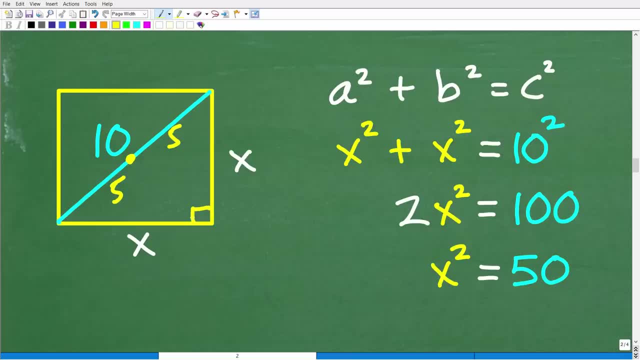 So our entire hypotenuse is 10, and this is a right triangle. What we can do is use the Pythagorean theorem. All right, So that's, a Square plus B squared is equal to C squared. Now, if you're not familiar with this, this is, uh, one of the most important formulas in all of mathematics. 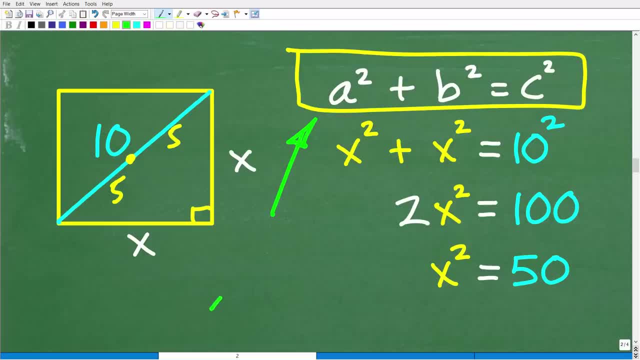 Really, I'm not really kind of exaggerating as well, but anytime you see a right triangle, that's a very poor triangle. Anytime you see a triangle and you have a 90 degree uh angle, uh as one of the angles in that triangle, you need to immediately think of this right here, which again is the Pythagorean theorem. 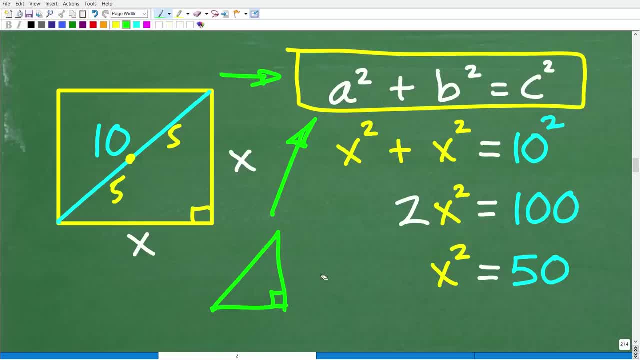 Now, what, uh is the Pythagorean theorem? Well, this basically equates the sides of a right triangle. All right, So the two smaller sides are um, are going to be A and B. The longest side, which is the hypotenuse, is always C. 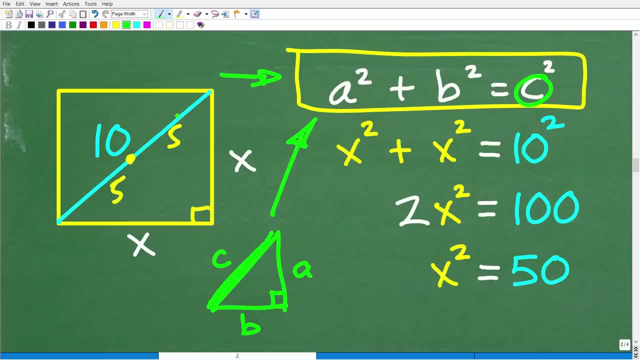 Okay, So C is always the longest side, the hypotenuse, and that's opposite of the 90 degree right angle. Okay, So visually too you can kind of see- that's pretty obvious- what the hypotenuse is. A and B can be the other two sides. 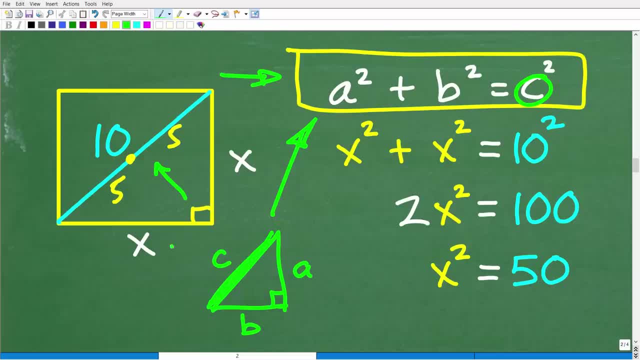 Now, in this particular case, Okay, Um, because our sides are X and X, it's like A and A. these are the same distance, but if we had uh different, um, uh lengths for our right triangle, then one would be A and one would be B. 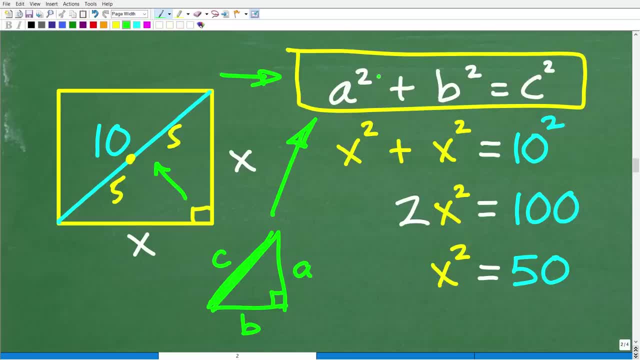 But basically the Pythagorean theorem states is that if you square the sides of the smaller sides and add them together, it's going to be equal to the square of the hypotenuse. All right, So let's use this Pythagorean theorem to figure out this side of this um. 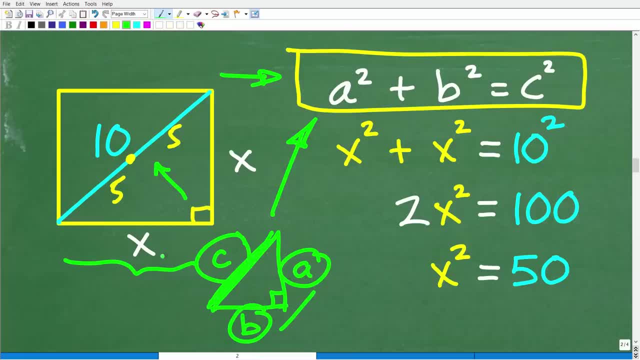 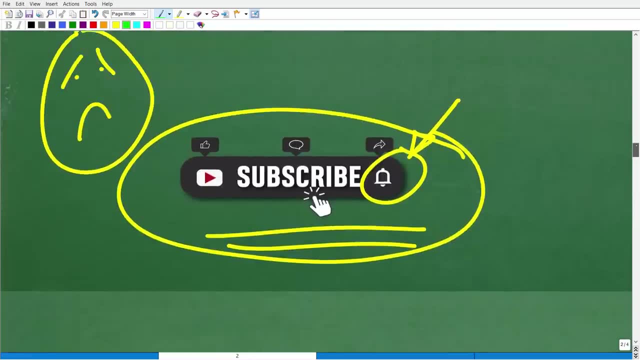 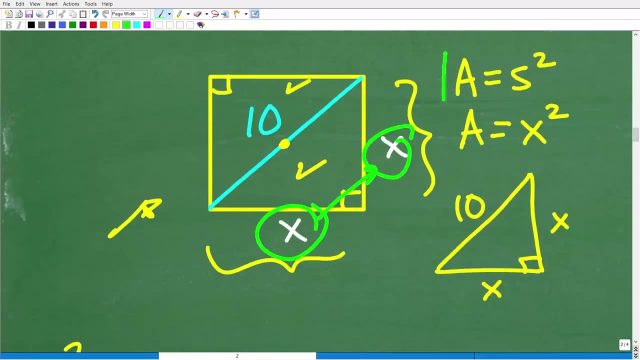 uh square here. Once we have this uh side, then we can calculate the area, right, Okay? So remember, okay- I'm going to kind of go back here because this is going to get quite interesting- is that the area of this square is what it's? X times X, right. 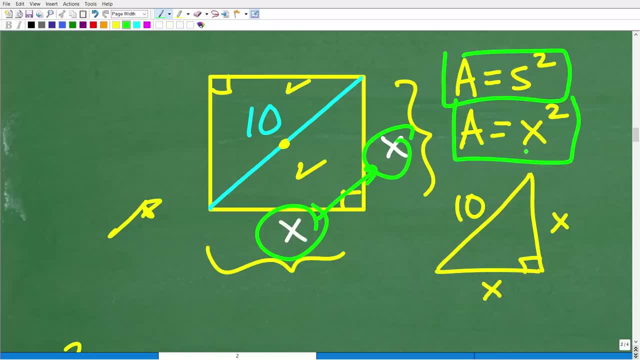 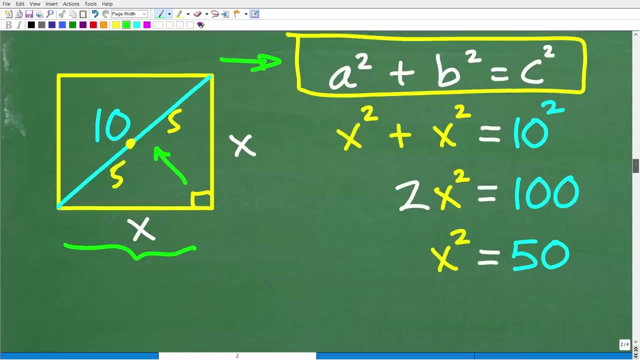 So, uh, X is the side, So we can figure out what X squared is. Well, that is indeed, is the actual area of the square, which is answering the question. All right, So let's go ahead and get into this right now. 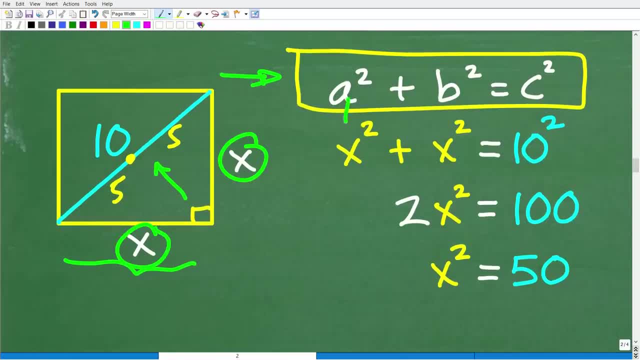 So our side, It's our X and X. So this is going to be X squared for a and X squared for B, and that's going to be equal to our hypotenuse, which is 10 squared. All right, So X squared plus X squared is equal to 10 squared. 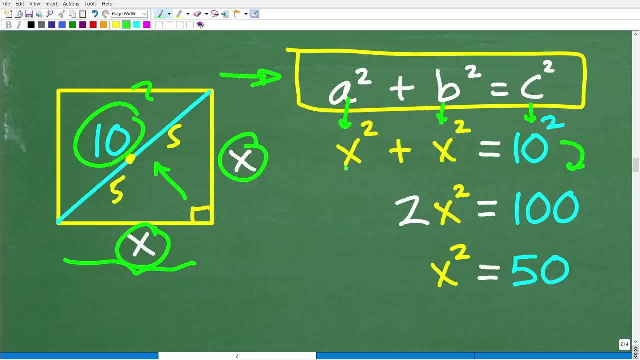 10 squared is 10 times 10 or 100.. And here I have X squared plus another X squared. I have two X squared, right? So two X squared. So now I'm on my way to solve for X. This is a quadratic equation, uh, cause I have an X squared but I don't need to actually do the uh uh. 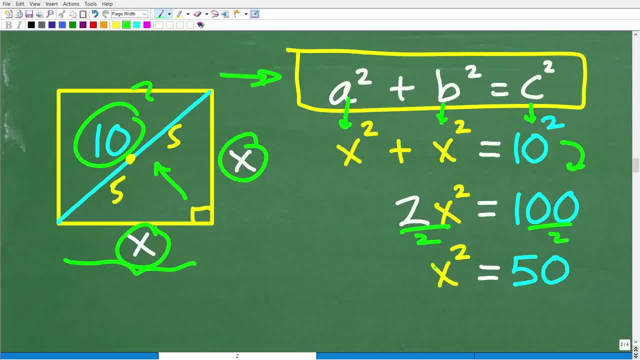 the entire problem, because when I divide both sides of the equation by two, I get: X squared is equal to 50.. And here I can stop, because I'm like, oh wait a minute, I'm looking for X squared, because X times X is the area. 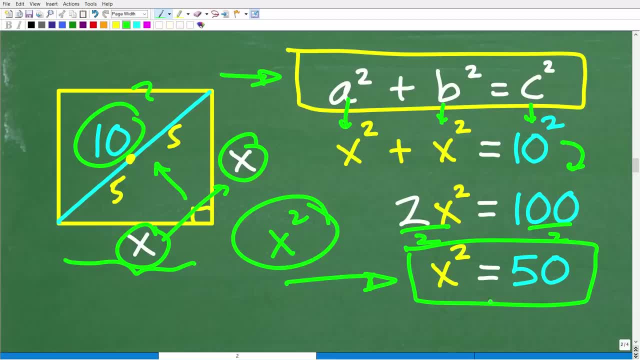 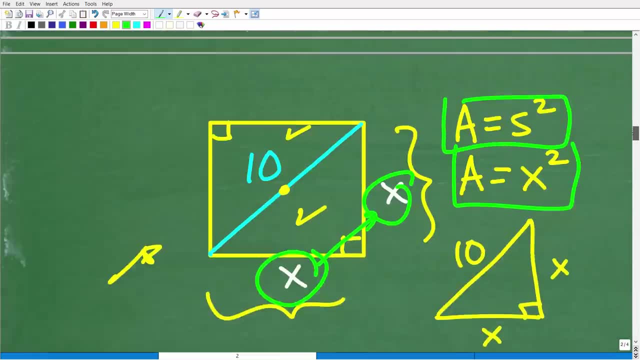 So X squared, indeed, is the area. So the area of this square is 50 units squared, All right. So again, uh, you know, um, hopefully, probably, um, you know most of you, this is like really kind of all. 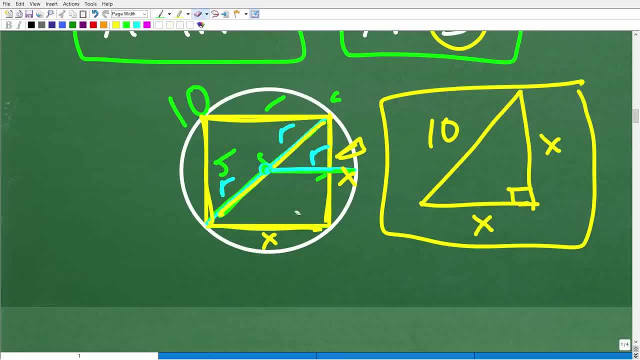 Written up here. but the most challenging part of this problem, in my opinion, is really kind of seeing that the radius here- let me kind of erase all this right here- uh, just so we can kind of see a little bit better that the radius when you look at our circle here is our square. 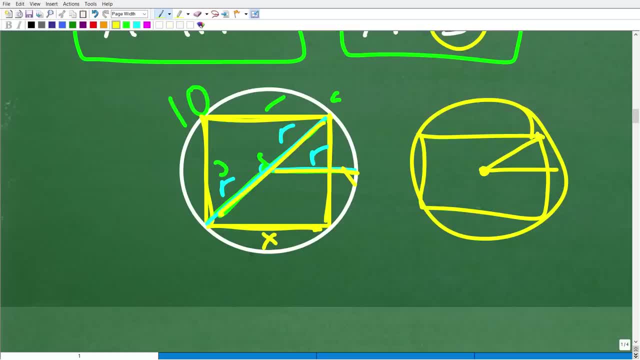 And you think about the radius, you're like, oh, it's out to here, but it's also along the diagonal as well. So that's really the key to unlock this problem. So that was like the first thing you needed to know.